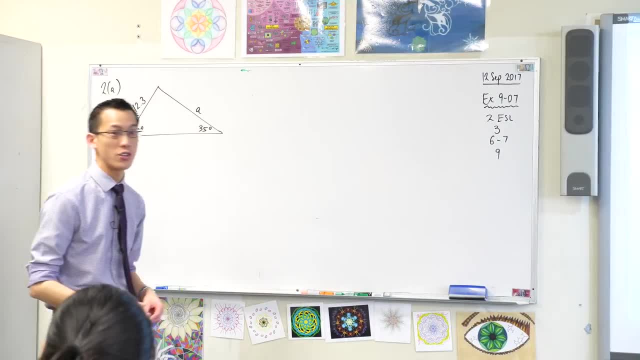 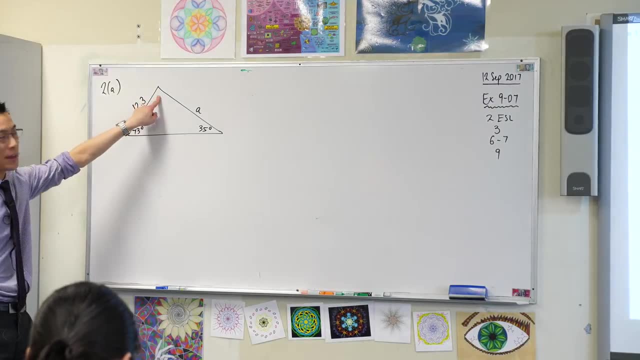 Is this the kind of question we're used to encountering in trigonometry? What's missing? A right angle? There's no right angle in sight, and there's an angle up here which you think, oh, maybe that's a right angle, but it's not. 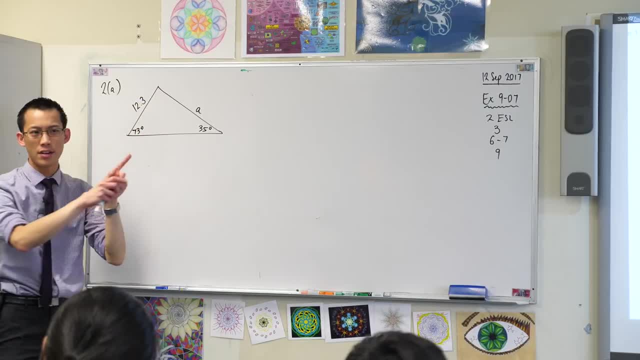 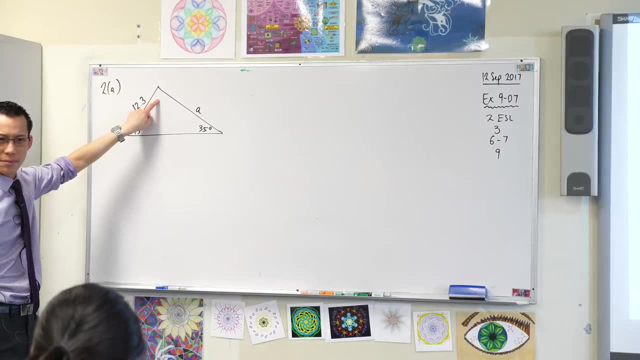 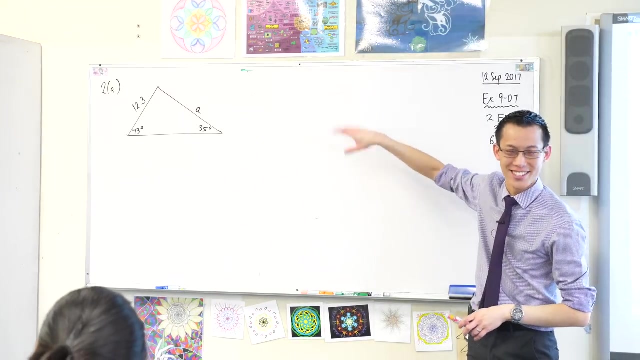 Have a look: You've got 73 and 35.. That's 108.. That makes that 72.. This is no good. Now, yeah, why is that? Yeah, yeah, I'll get to the title in a minute. You can see I've left it off intentionally. 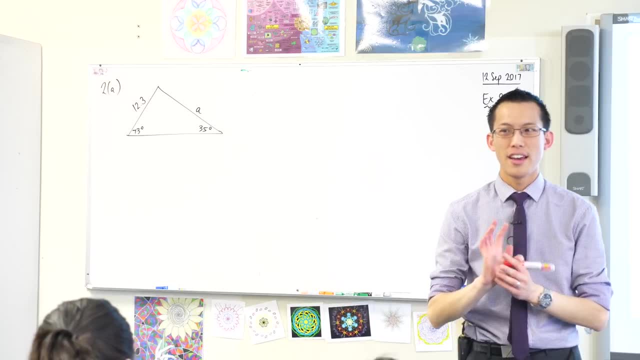 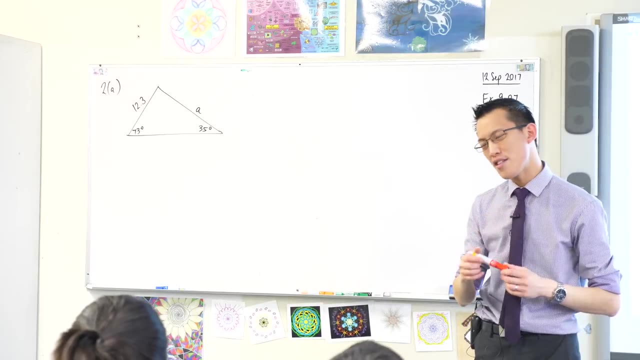 Now, shh, shh, shh shh. There's no right angle in this triangle, so therefore, I'm going to find it really hard to use trig, because all of the things I know about trig so far have been to do with right angle triangles. 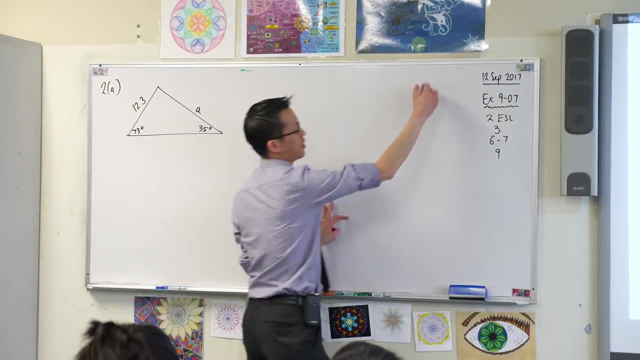 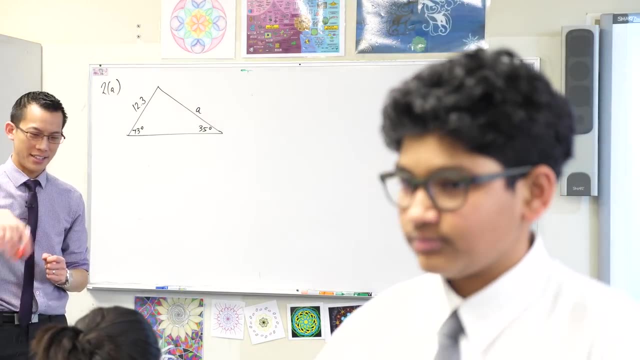 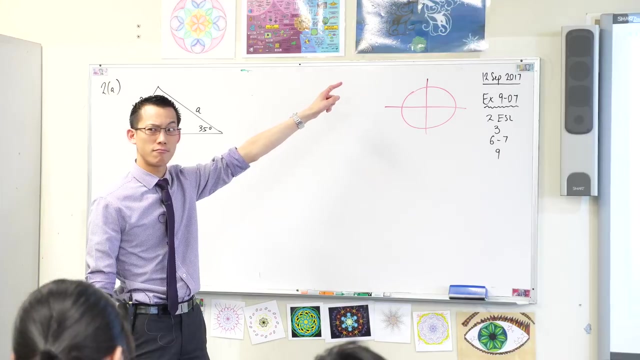 Well, yeah, that's right. Now, here's the thing. Don't draw this, because you've already got this. We found trigonometry in the unit circle. by doing what? What did we do? We drew a triangle. We drew one there. so we're like there's no right angle triangle, No problems, Just put one in right. 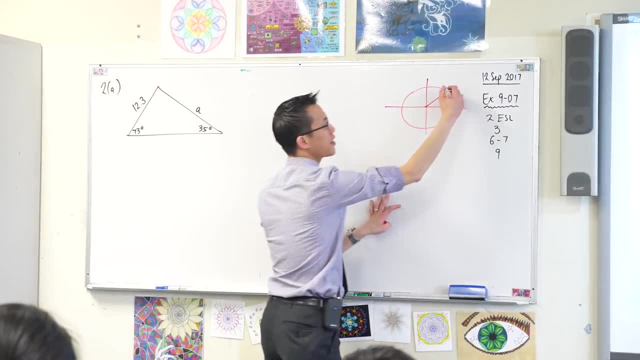 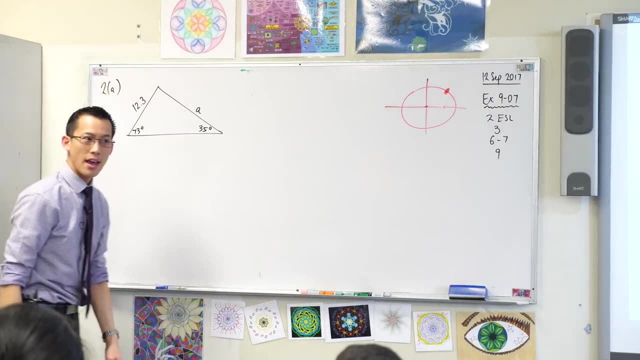 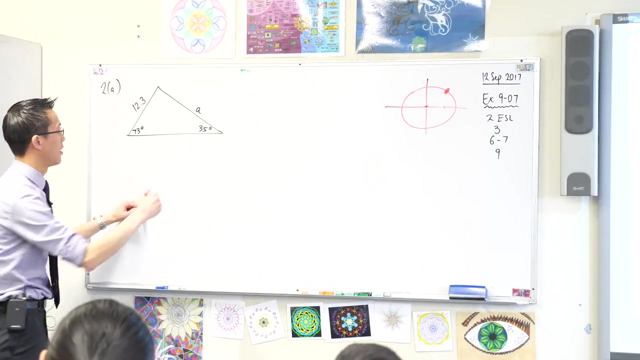 And then, once you work everything out, then you're like: oh, don't worry, Now that I know what this point is, I can forget that the triangle was there. I can hide it, as it were. Now see, this triangle is not right angled, but I'm going to put a right angle triangle in it. In fact, I'm going to do two. 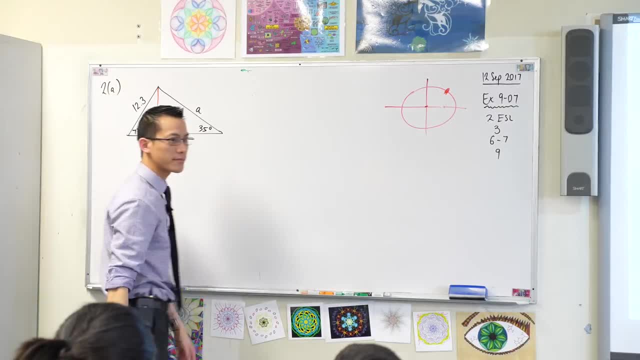 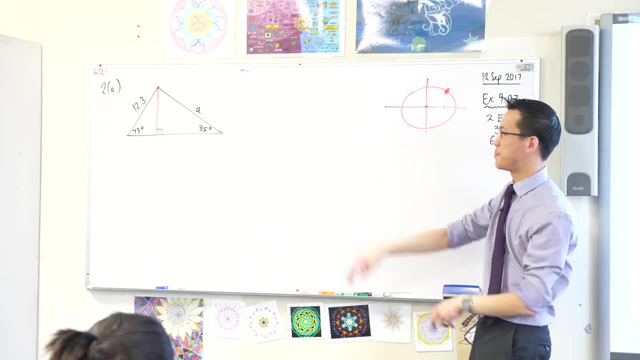 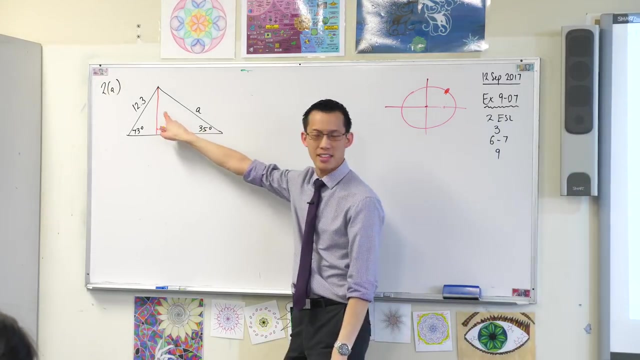 Can you divide this triangle down like this? Okay, Now, this is why I asked you to sort of rotate it around, just to make this bit a little bit easier. Now, you might think that that's a bit of a step backwards, because I don't know what this length is anyway. so how is it useful to me? 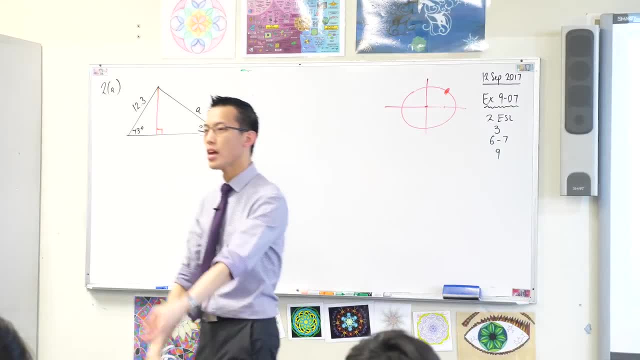 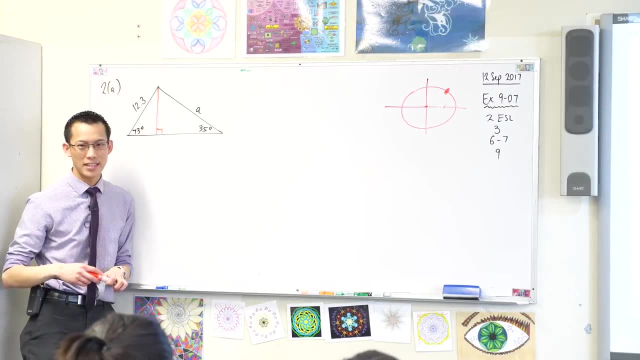 Well, just watch and see. okay, I don't know what this length is. Stay with me, E10.. I don't know what this length is, But thankfully I have a whole field of mathematics that deals with numbers that I don't know what they are. 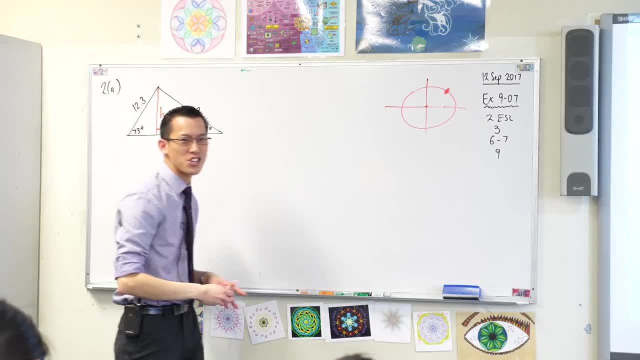 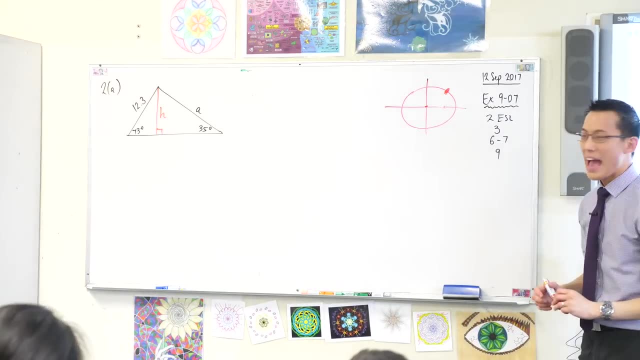 Algebra. I'm just going to call this guy h. Why do you think I call it h? That's how tall it is okay. So I'm just going to call it h for height. And once I have that number there, that pronumeral, I should say this is the brilliant part. 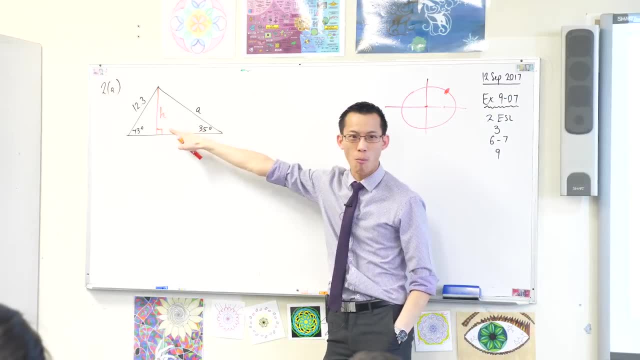 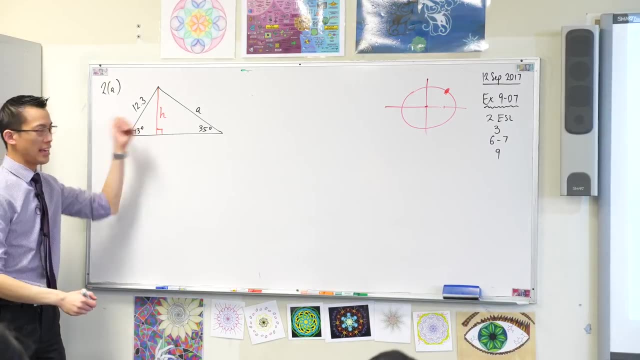 I'll never find out what it is, but I don't need to. I just use it there to help me out for the number I really want. Okay, Watch this. okay, Have a look at this left-hand triangle over here, This little triangle with a 12.3 and h and 73.. 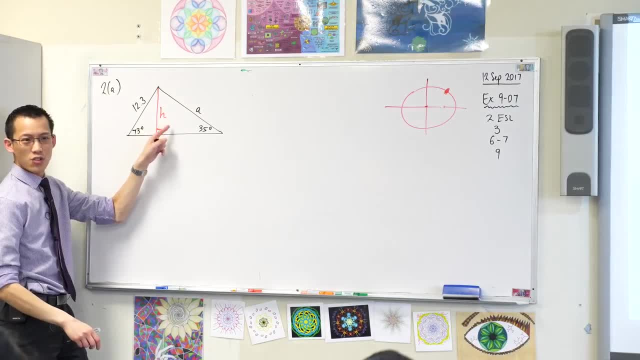 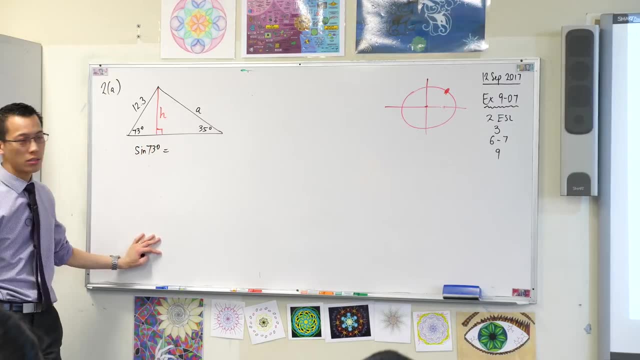 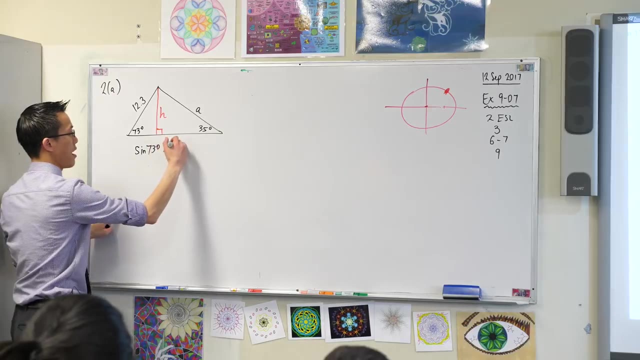 Okay, I can say in this triangle that sine of 73 degrees is what? Have a look, Because it's a right-angled triangle. right, It's opposite. on hypotenuse, Do you agree? h on 12.3.. 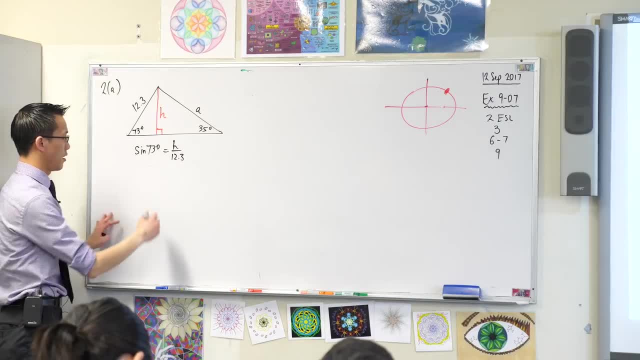 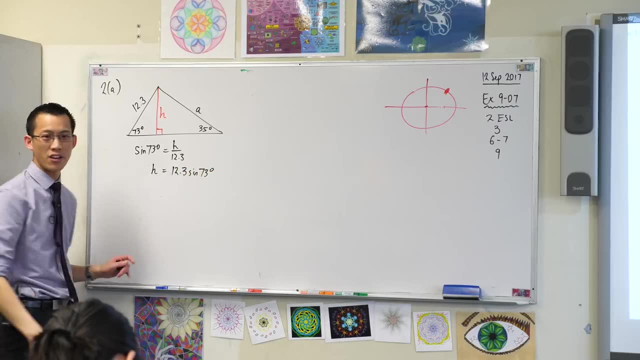 Okay, No big deal. I can therefore say that h is this: I'm just multiplying both sides by 12.3.. Is that okay? Now, if I wanted to, I could go ahead and I could punch that into my calculator. 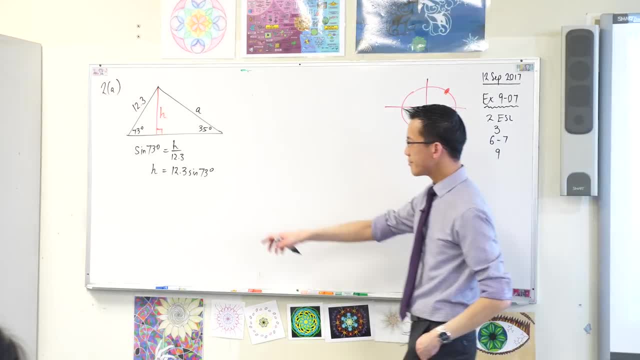 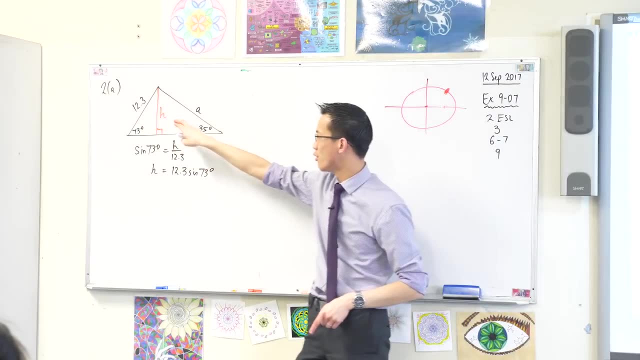 But watch this, I don't need to. Okay, See this. See this. It's from this triangle on the left-hand side, right, But look, there's another triangle on the right-hand side which also has h in it. Okay, 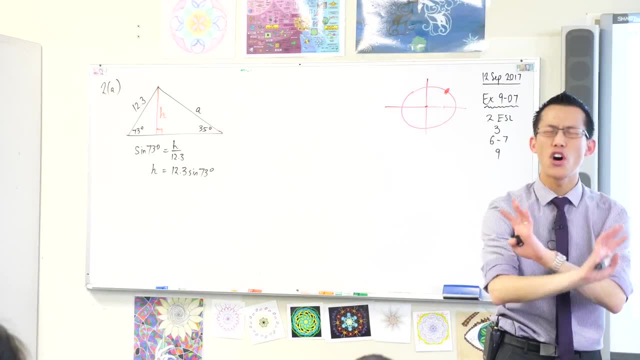 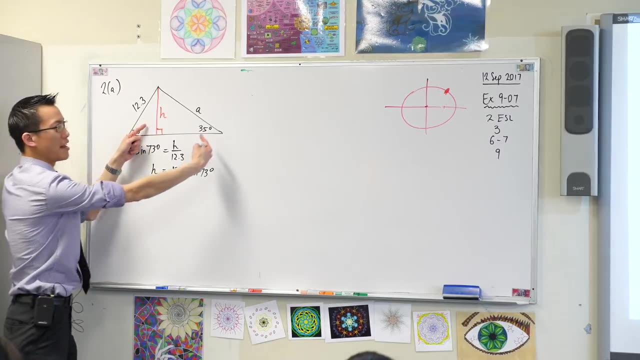 So what I'm trying to do here, This is the skill. It's not about the number, It's about what's happening in your brain. Okay, I can look at the same object from another point of view and get more information about it. Watch. 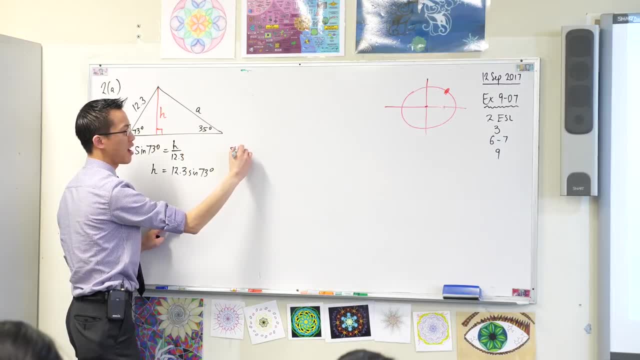 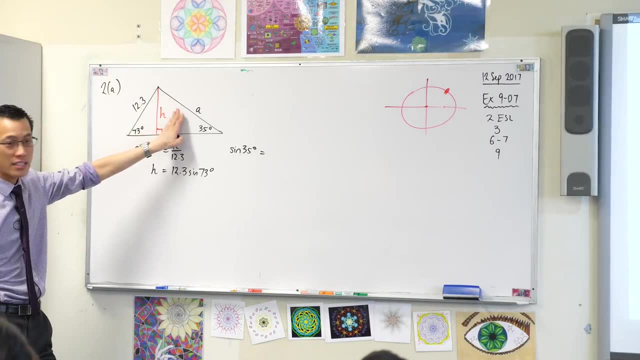 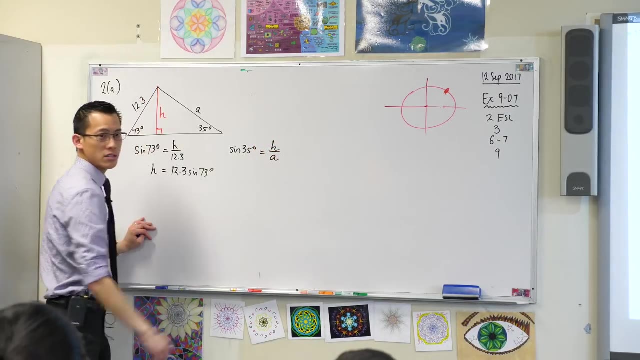 In this triangle. I can say: sine of 35 is what? Look carefully, This is the right-angled triangle, Just this one over here. Isn't it? opposite on hypotenuse, Opposite on hypotenuse? Do you agree? 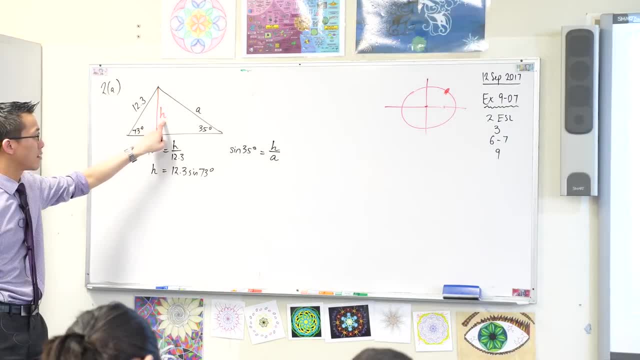 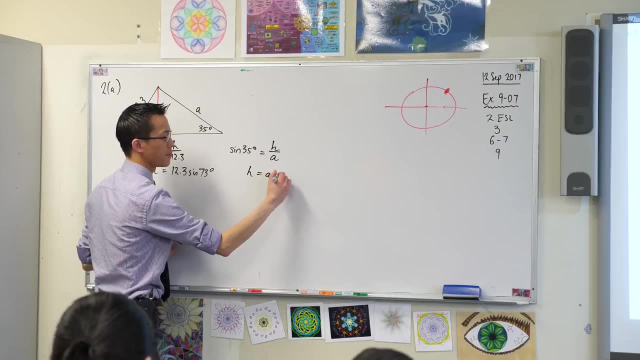 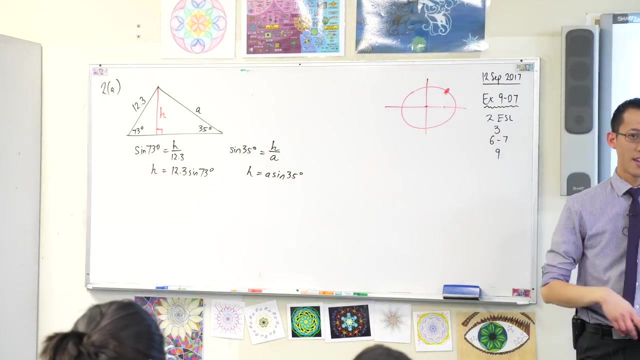 Do you see it? Opposite 35 and hypotenuse of this triangle. So now I have this. Does that make sense? I've just multiplied both sides by a. How's your brain doing? Okay, Two right-angled triangles.